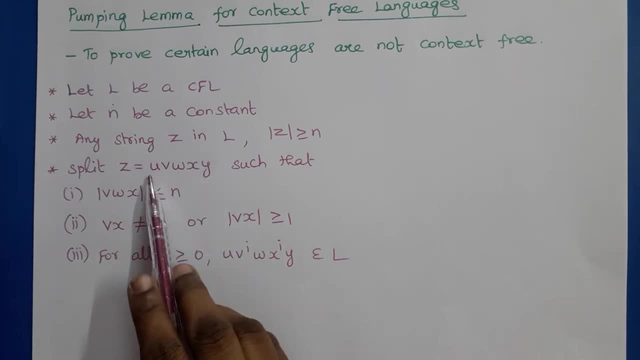 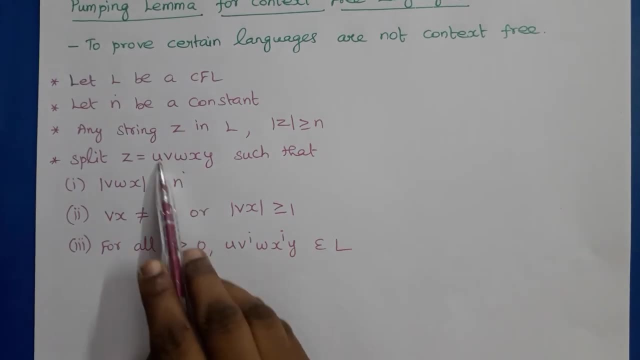 Z into five substrings, uvwxy, such that it should satisfy these three conditions. the middle portion, vwx. length of the middle portion must be less than or equal to this constant n. okay, the length of Z total length length of uvwxy must be greater than or equal to n in which this vwx. 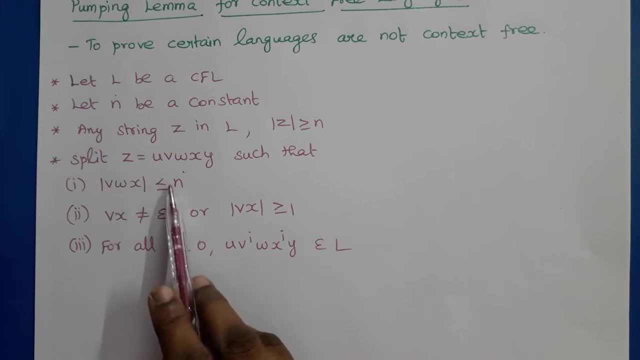 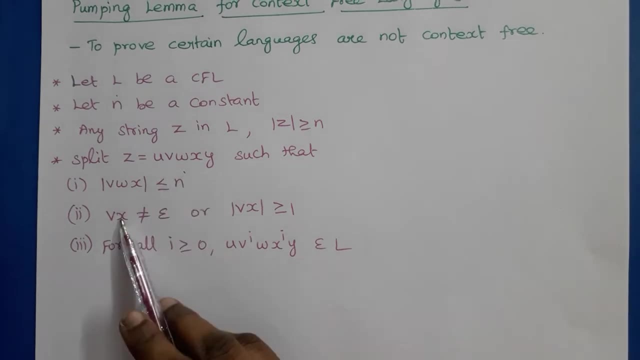 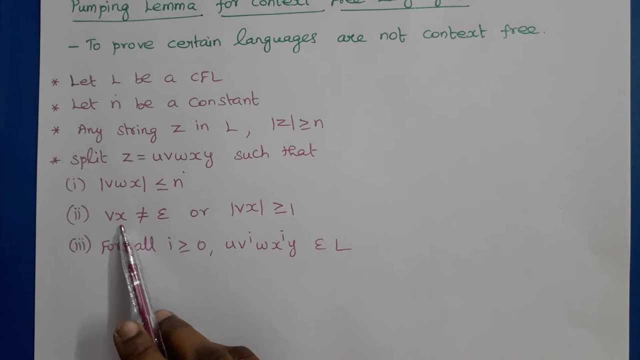 the middle portion portion's length must be less than or equal to n maximum of n. It can have maximum of length n. Then this v and x. okay, this v and x. that means here we are going to pump v and x. So this v and x not equal to epsilon. The meaning is at least v or x must contain one. 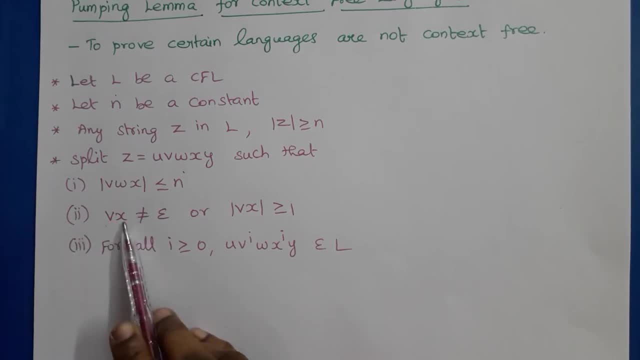 symbol, So vx. the concatenation of vx is not equal to epsilon. or we can also say that length of vx is greater than or equal to 1. So at least its length is greater than or equal to 1. So 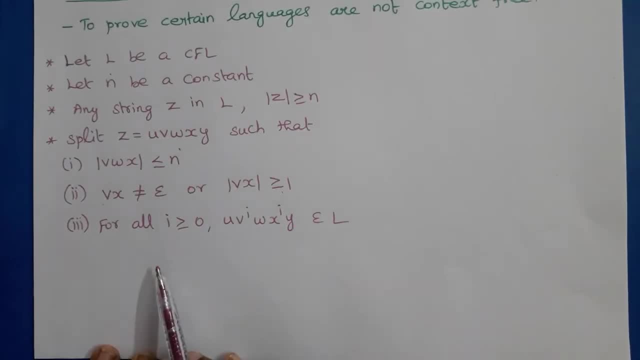 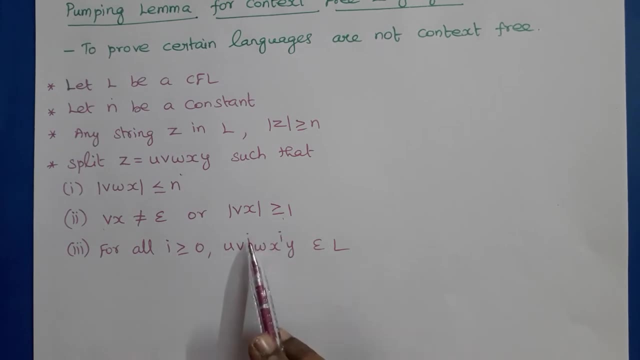 at least one symbol must be present. Then we have to prove for all i greater than or equal to 0, that is, if we pump v and x means u? v to the power i x, sorry, u v to the power i w. 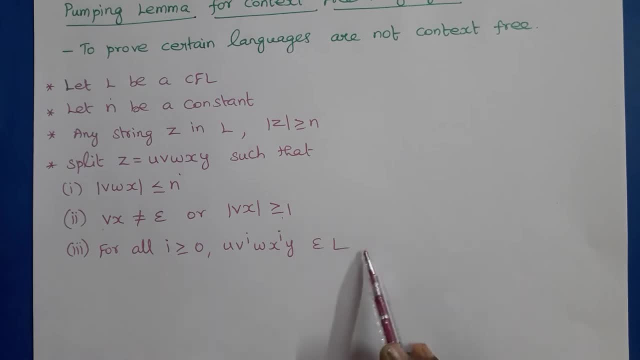 x to the power y should also belong to n. so if we pump v and x i times, including 0 means the resulting string must also be in the language n. so it should be proved for all i greater than or equal to 0. sometimes the string may be true for some few i values 0, 1, 2 etc. so in that case we can prove. 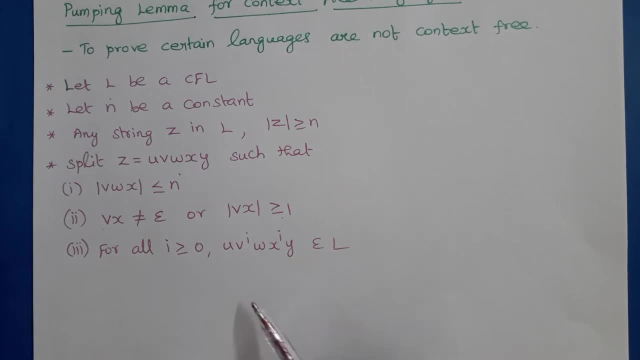 prove it, for i equals 3, so the condition is: for all i values greater than or equal to 0, the string must also belonging to l, so we will get contradiction here, so we can say that the given language is not regular. so pumping lemma is used for proving. 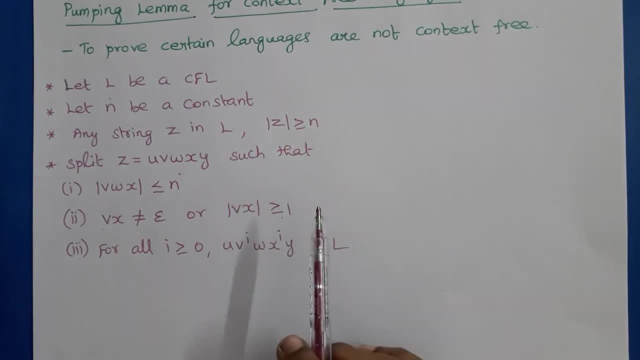 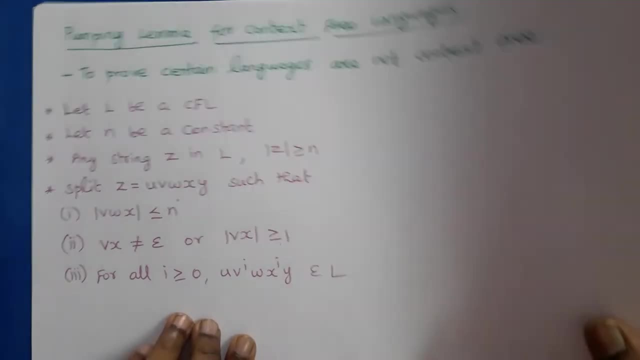 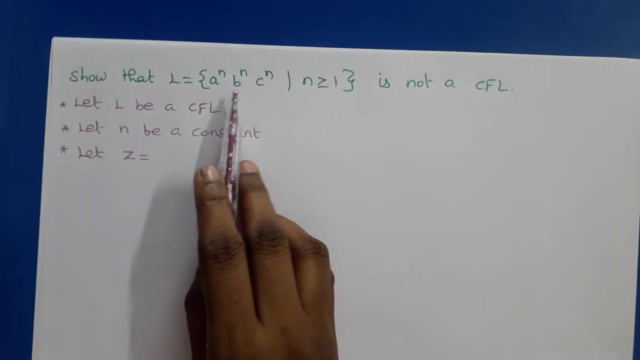 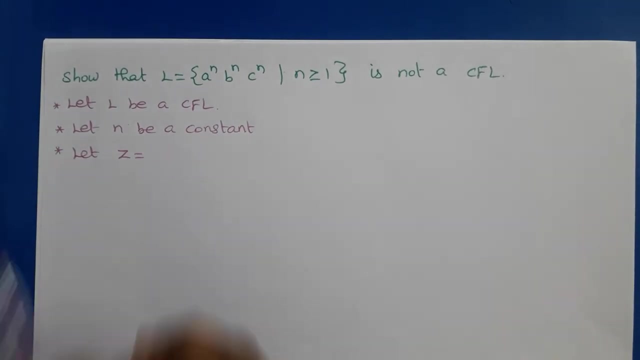 the language is not a context free. it is not used for proving a languages. language is a context free. now we will see an example. so show that l is equal to a to the power n, b to the power n, c to the power n, such that n is greater than or equal to 1, is not a context free language. so consider: let l be a cfl. so first, 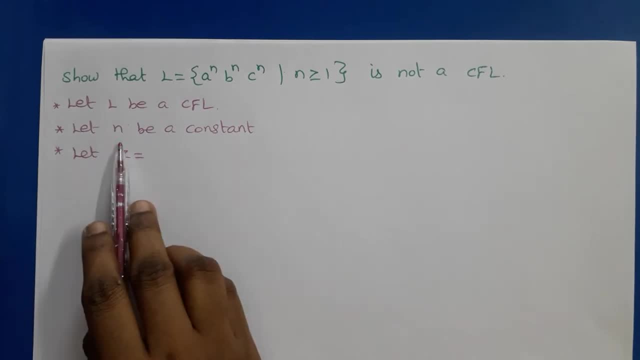 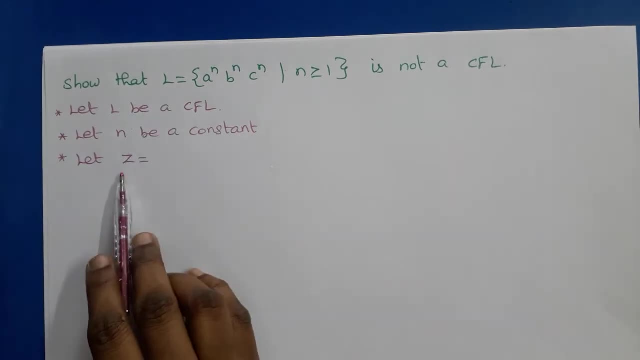 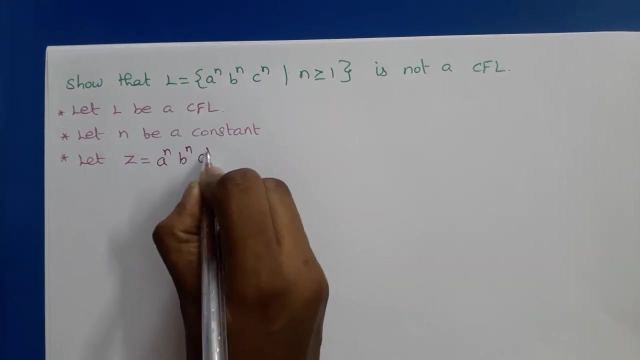 assume that the given language is a context free language, then let n be a constant. this n be a constant. now we need to choose z belonging to this language, l, so z choose z. equals a to the power n, b to the power n, c to the power n, so n number of a's must be followed. 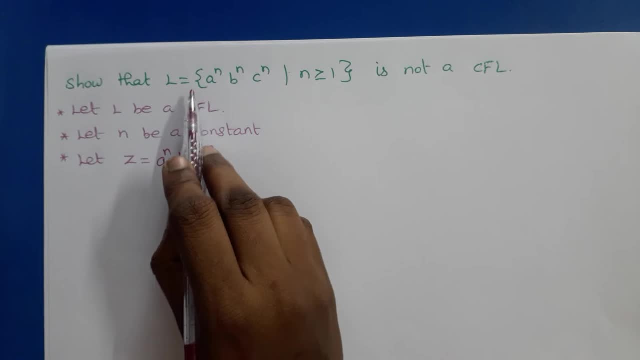 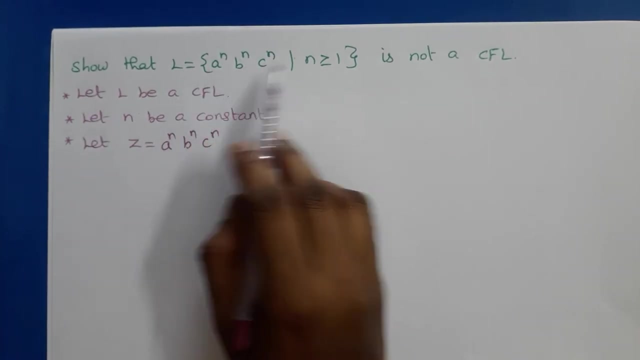 by n number of b's followed by n number of c's. actually, for this language we cannot construct cfg right, we can construct cfg for a to the power n, b to the power n, but we can't construct cfg for a to the power n, b to the power n, c to the power n. so we can prove it's. this language is not a cfl. 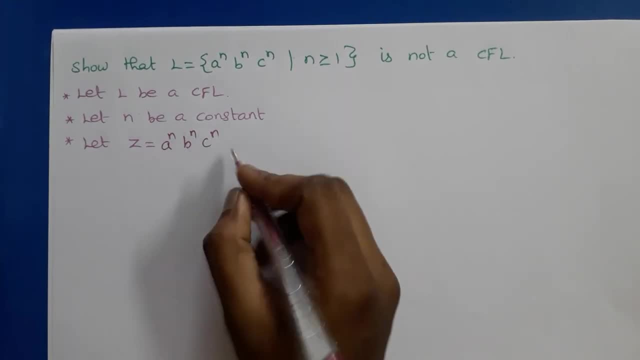 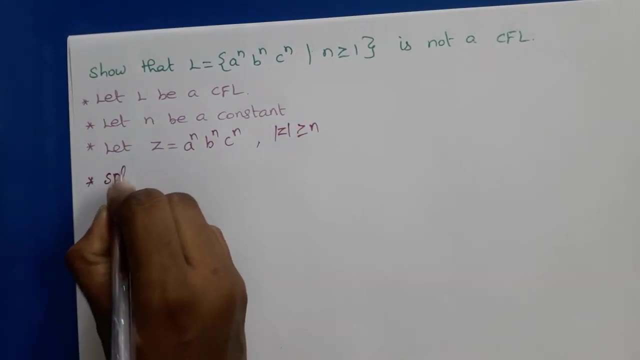 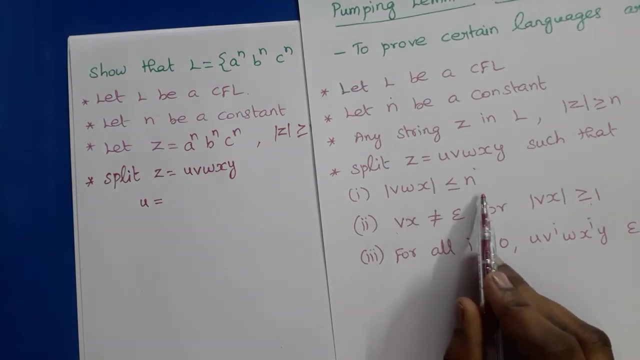 using pumping lemma. so z equals the string, such that length of z is greater than or equal to n. it satisfies this condition. now split: z equals u, v, w, x, y, in which u equals. actually, the first condition is v w, x is less than or equal to. 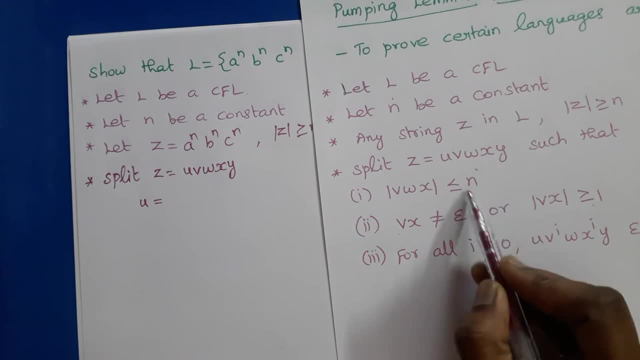 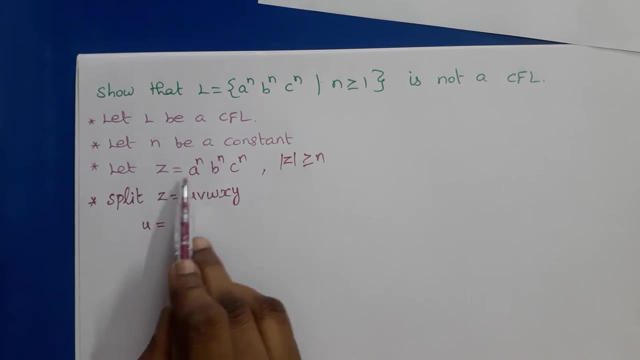 n. right. the middle portion is less than or equal to n maximum of n. so we can consider v, w, x as b to the power n. so we can assign a to the power n to u and c to the power n to y, so u equals a to the. 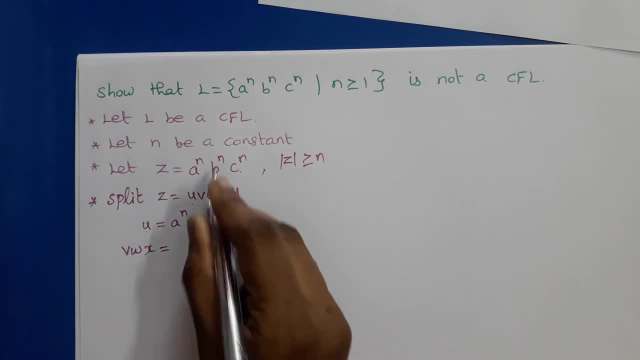 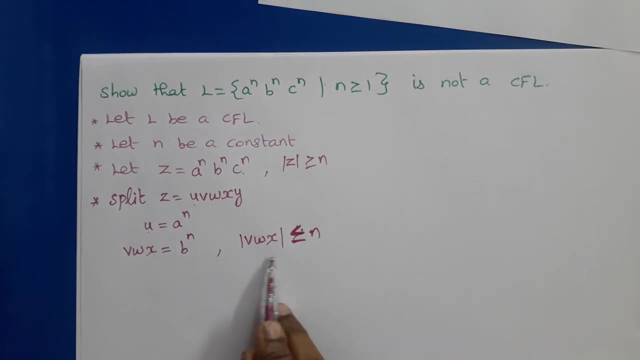 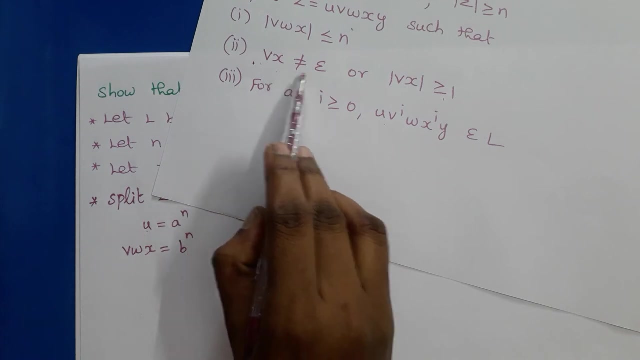 power n, v w x equal to b to the power n, such that length of v w x must be greater than or equal to- sorry, less than or equal to n. length of v w x is less than or equal to n. now the next rule is: v x is not equal to epsilon, that is at least. length of v x is at least one right greater than or equal. 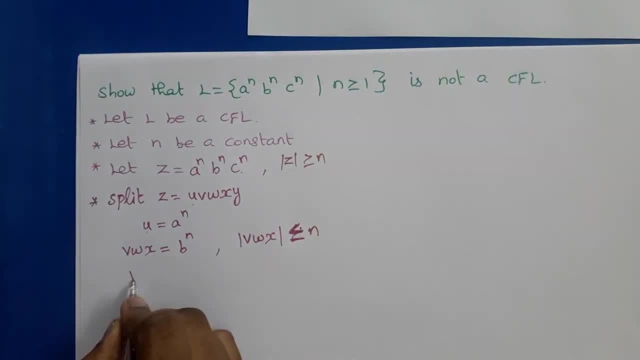 to one. so v x from v w x, we can choose. v x, v x is equal to b to the power n minus m. that is, we are going to assign some b to the power n minus m number of b's. some n minus number of b's are. 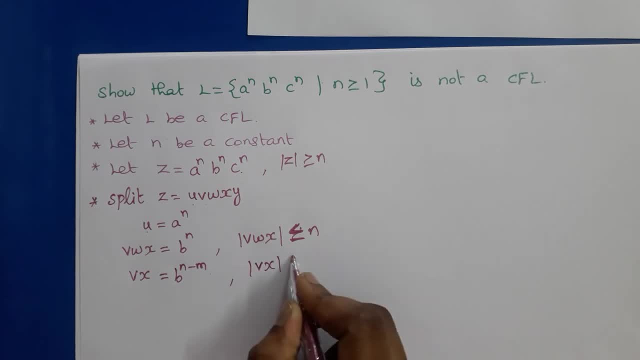 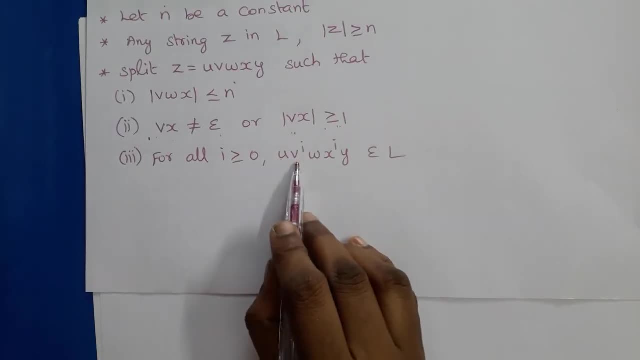 assigned to v x, because length of v x must be greater than or equal to n. so v x is less than or equal to 1. then we need to prove u v to the power i, w x to the power of i. y belongs to l, so 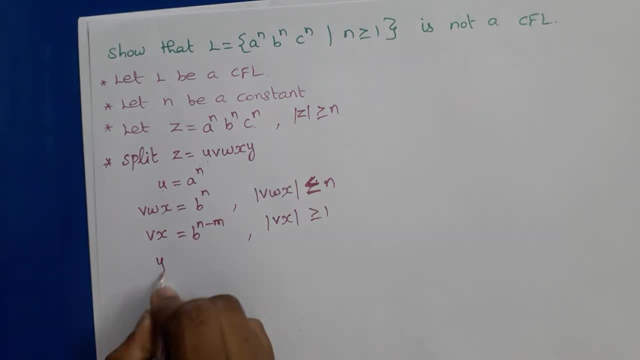 and here y is c to the power n right. so we have splitted z in the form of u, v, w, x, y, and a to the power n is assigned to u, c to the power n is assigned to y, b to the power n is assigned to. 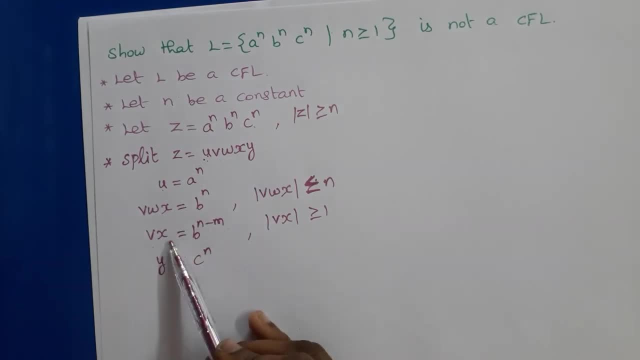 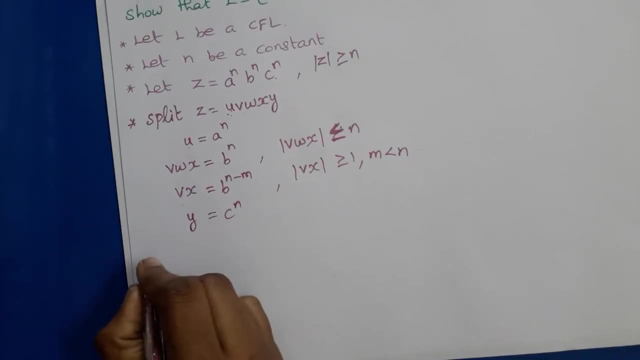 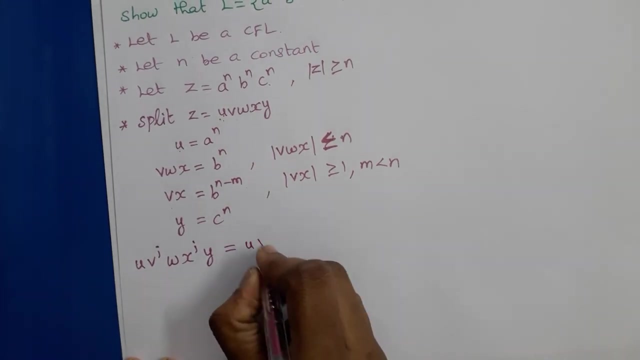 n, and here n minus m is assigned to b to the power x, and here we can also say that this m is less than n. okay, so now u, v to the power i, w, x to the power i, y, so this can can be written as u v, v to the power i minus 1, v can be written as v. 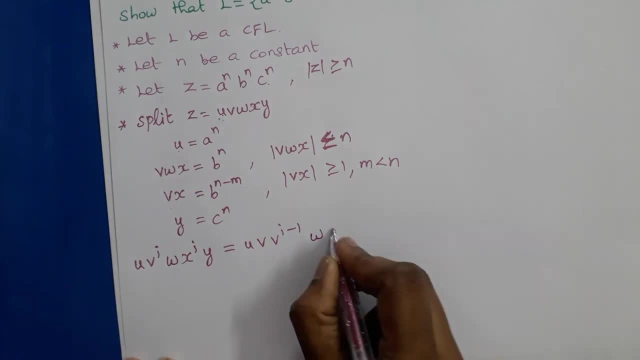 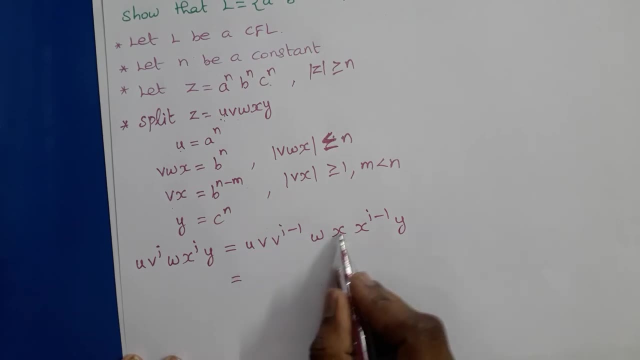 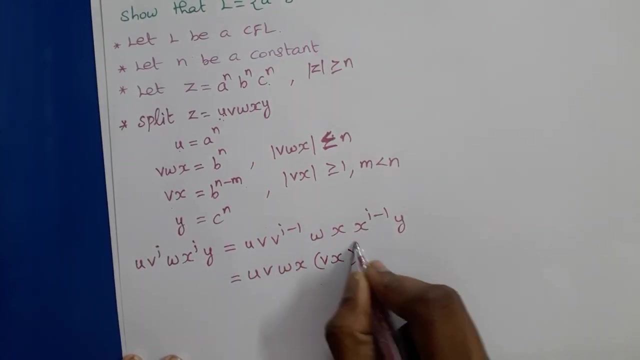 concatenated with v to the power i minus 1 w. similarly, x into x power i minus 1 y. now we can combine. we can bring w, x here, so u, v, w, x, and we can combine this v and x to the power i minus 1 y. now we can substitute values for these. 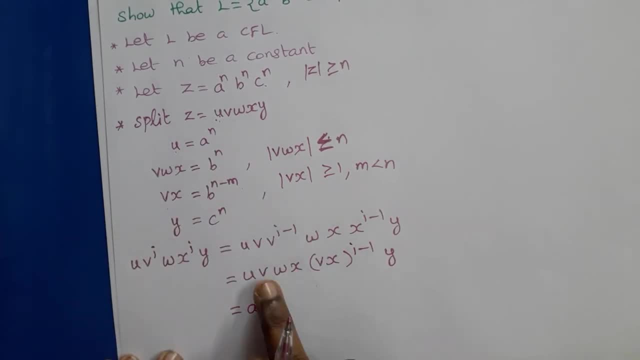 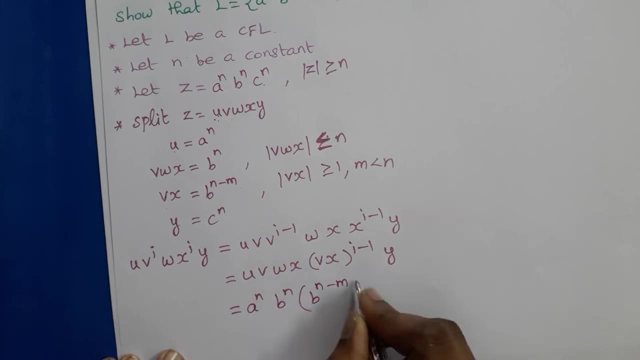 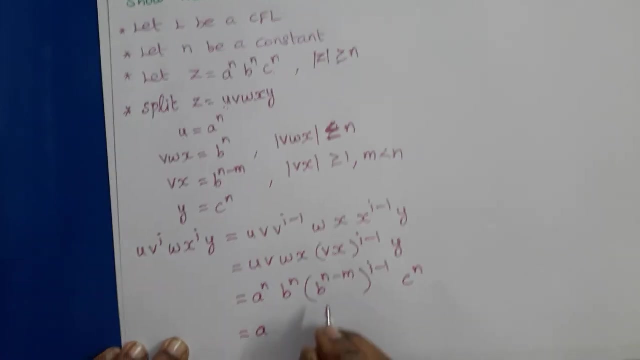 symbols. so u means a to the power n, v, w, x, b to the power n, v, x is b to the power n minus m, to the power i minus 1. okay, then y is c to the power n. so now a to the power n, b, power n.